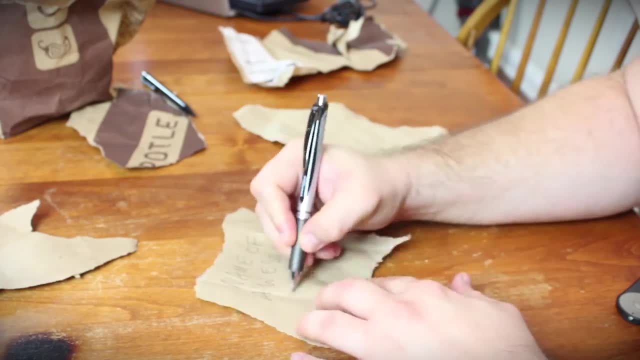 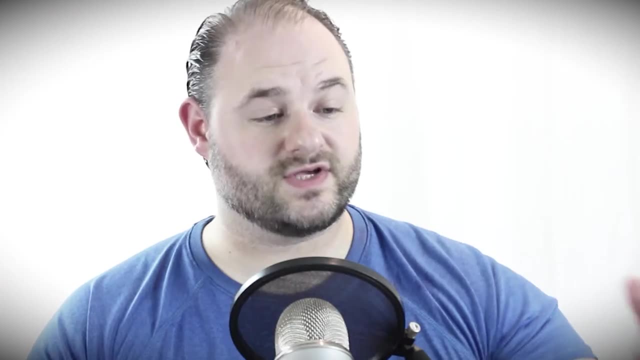 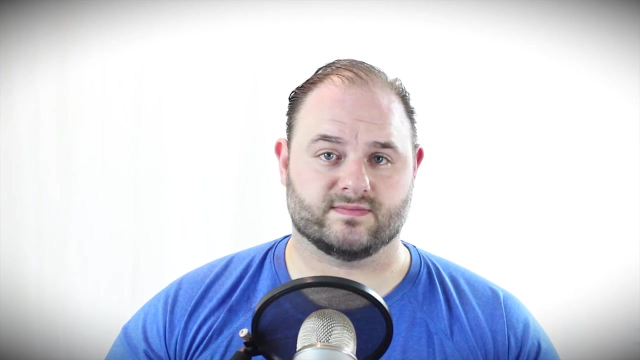 So as soon as you make up something like this, the quicker you're going to be able to play, And the quicker you can play, the quicker you can test things out to make sure this mechanic works and this mechanic doesn't. Or our dolphin versus manatee game is not as awesome as we thought it would be. 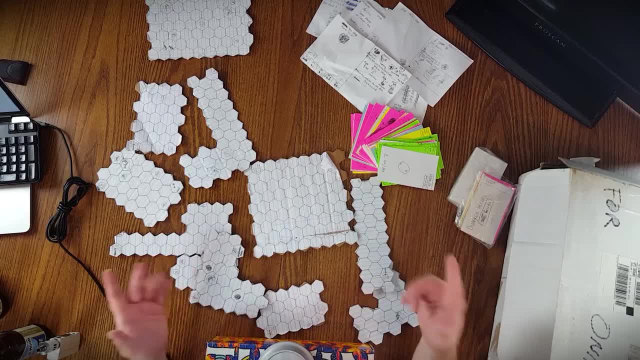 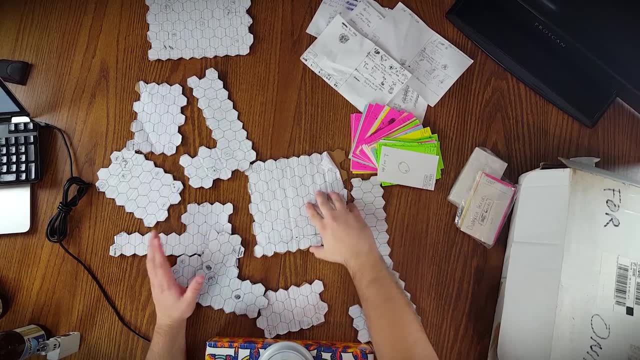 All right. so, as you can see, we're already at the table here and I have some components that I made a long while ago And they were very functional and they're not very pretty. I mean, look at that, Look. 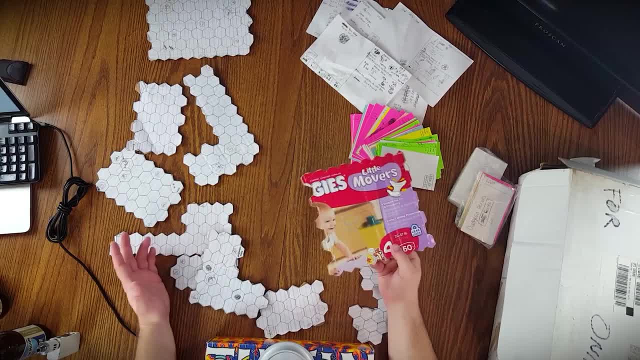 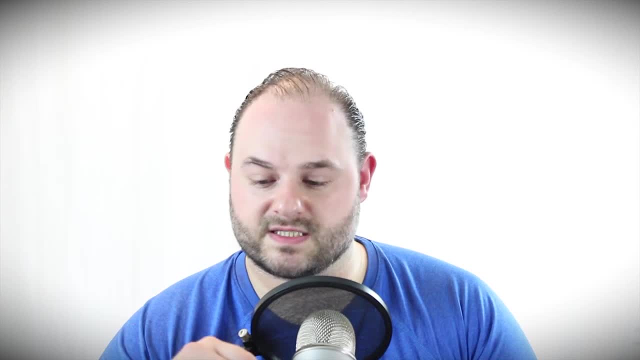 Huggies. All right, Yep, I made this game when one of my children was still in diapers. After a while you're going to think: oh man, I may as well add some stinking awesome illustrations on my junk. 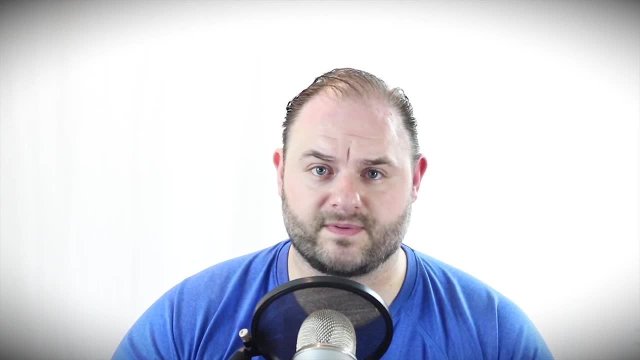 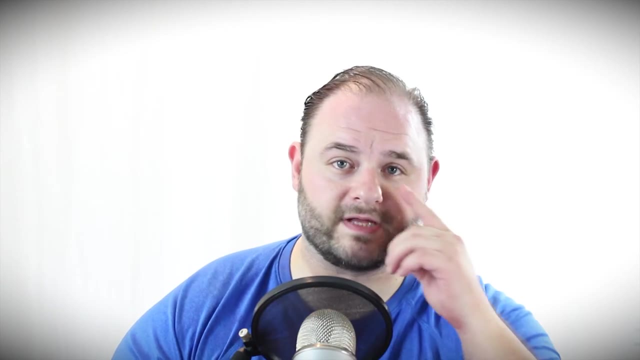 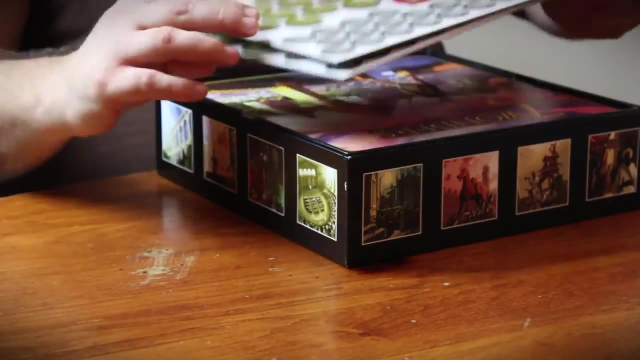 No Waste of time, Don't do it. The whole purpose of this step is not to really invest anything financially, but to test and make sure that everything's working. Now, other people like to go through and salvage things from other games, like dice, or, let's say, you find some cool little meeples. 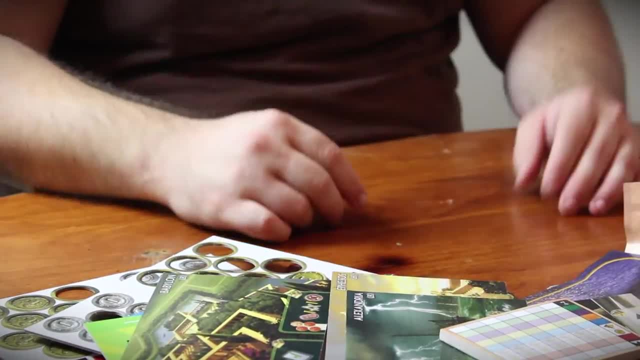 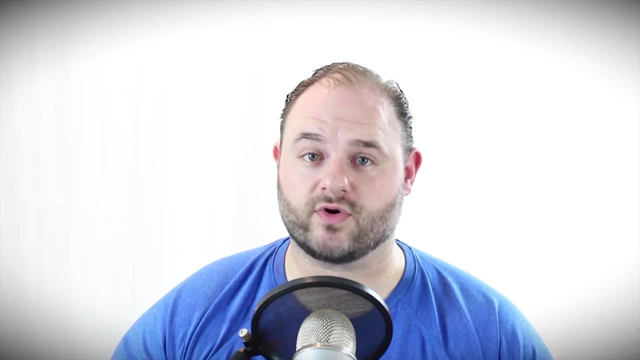 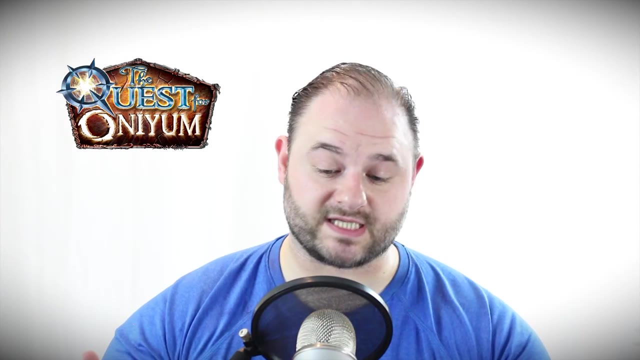 Use every bit of time that you can and use everything That you can find effectively. All right, so I know in our last videos we've been talking about Scribble Quest. Well, we actually already have another board game that's much further along than Scribble Quest, and I would just like to show you some of the components that we've been working on for the past several years. 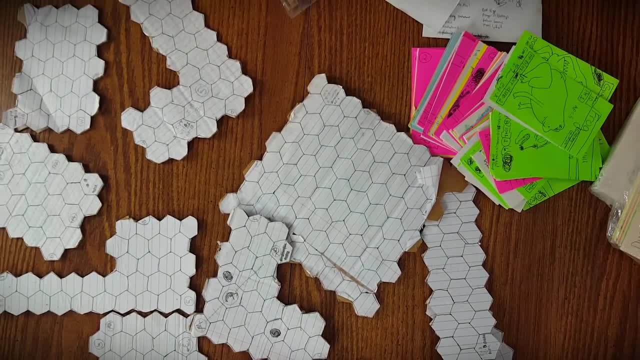 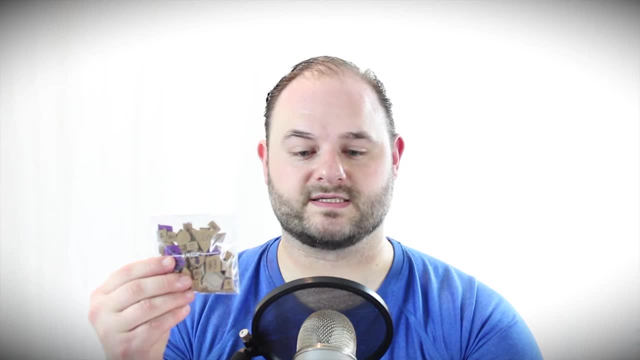 Now, as you can see, they're really not much to look at, and at one point I thought that nobody wants to write anything down. You can just use these little hit point counter things And you know what They were decent. 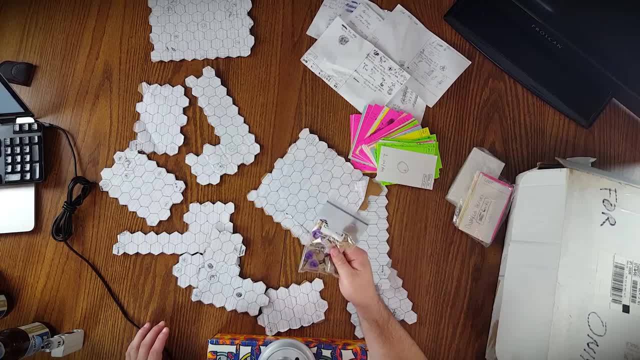 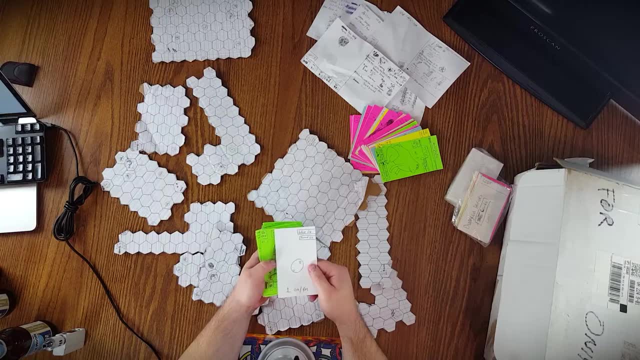 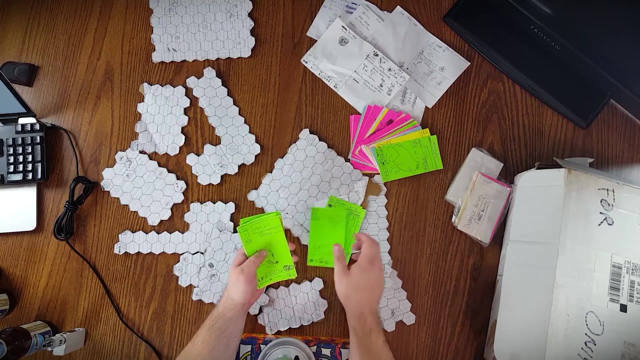 I think I maybe used them, but everybody else that we playtested with did not, So that kind of just went. yeah, Some other things that we have are three by five cards. Now I know that I'm an amazing artist. Whoa, that's a beautiful man, beast. 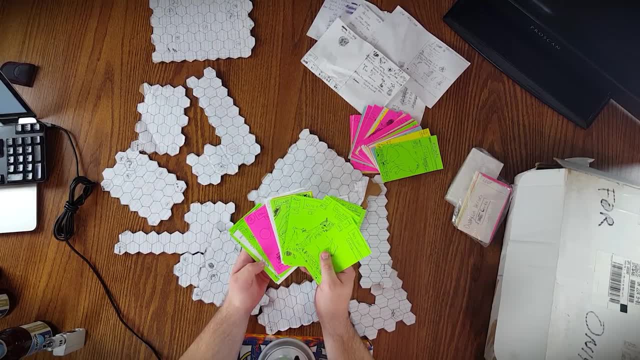 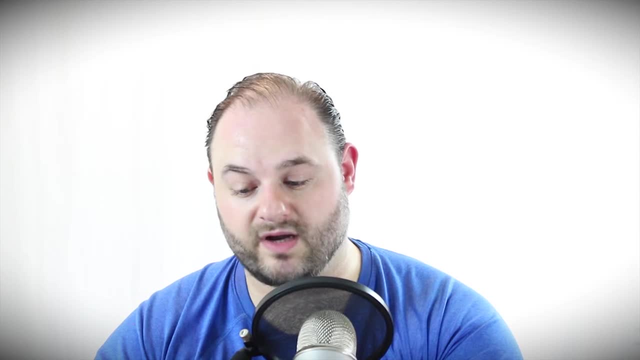 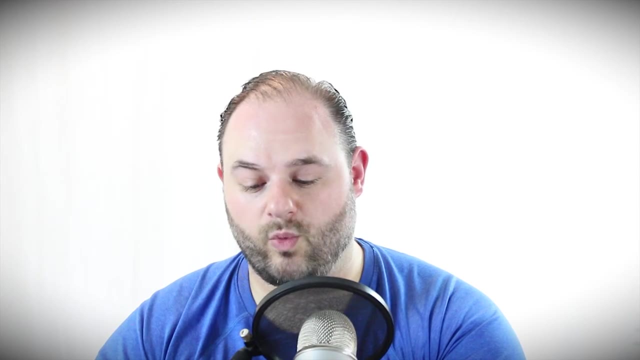 One thing that I did in order to test things out was also to test The way that these cards work. Now, these enemy cards were just one component of the game, and I kind of wanted there to be maybe not really a theme, but a way that you can distinguish the cards from the other cards. 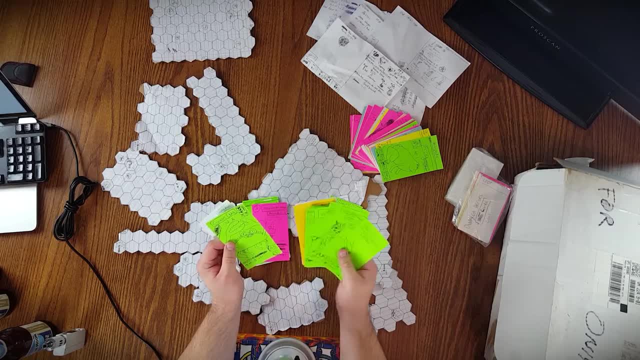 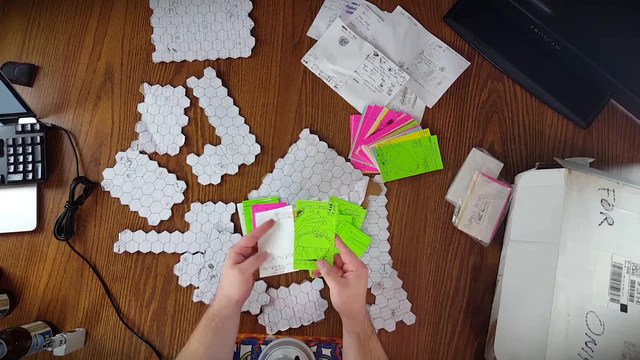 And actually, believe it or not, you would think that I had color coded them, but I did not. This was actually a reward card and this is an enemy card. Two different kinds of components, two different design cards And actually, 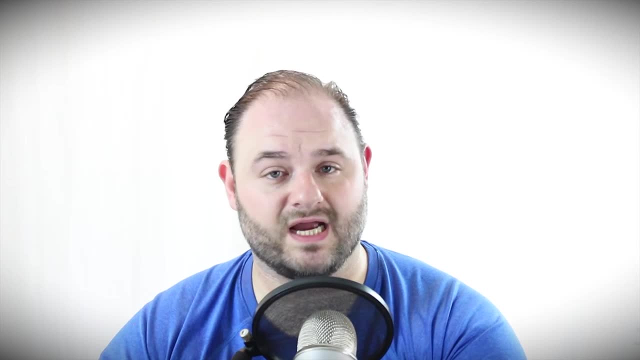 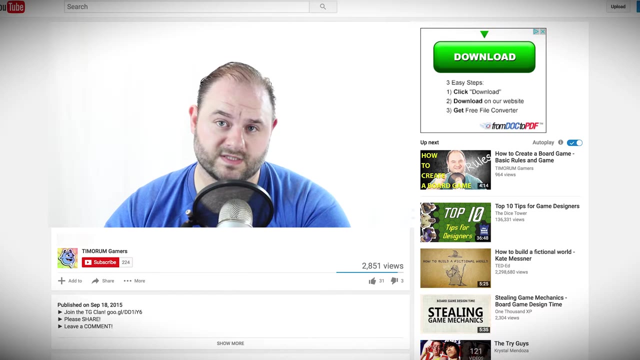 If you would like another video about the physical design of the components, then please let me know in the comment section down below. You know where it is. If you don't like, you must be new to YouTube. Hi, Welcome to YouTube. 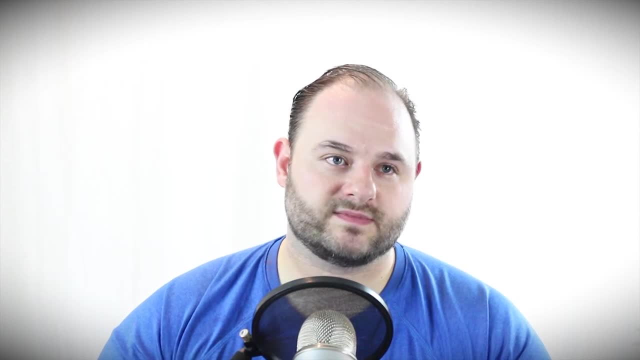 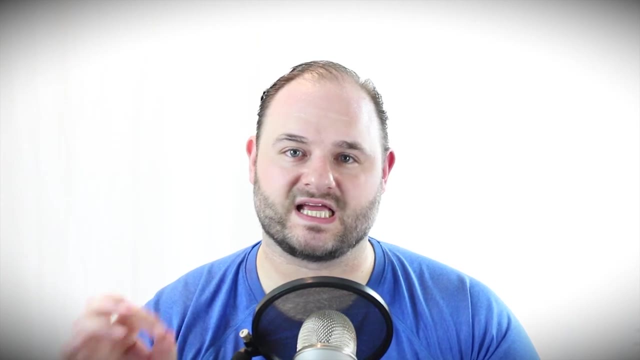 Prototyping is very simple, All right. But here's the deal. I kind of break it down into stages of prototyping, More like what is necessary just to get things going. I need dice, I need cards, Or I just need cards. 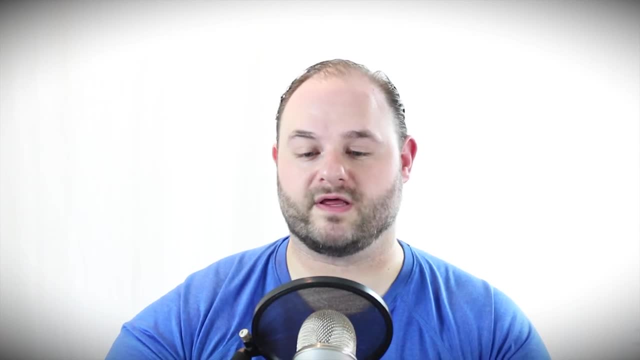 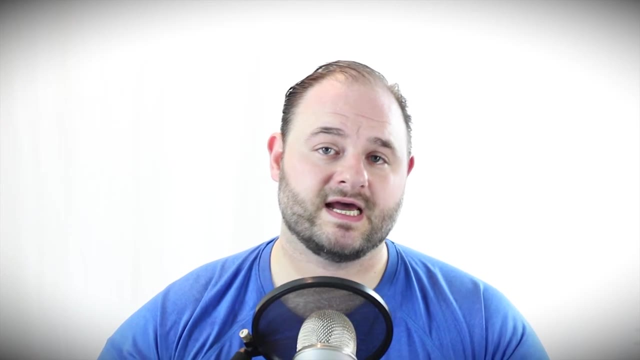 Or I need a game, Or I need a board, Any kind of component that you've salvaged and put together- and boom, you can throw it on the table to test things out. Now you can use that for several, several, several months. 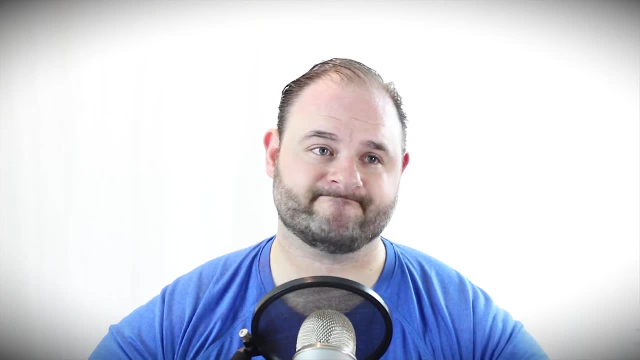 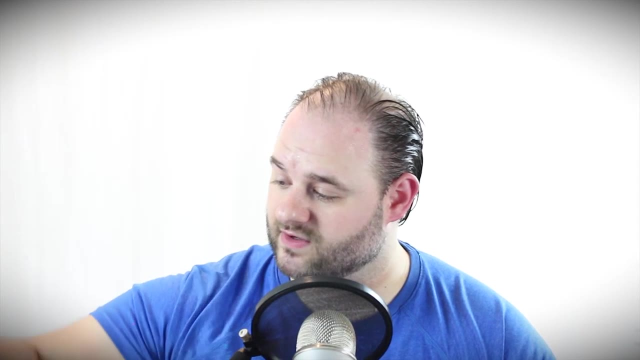 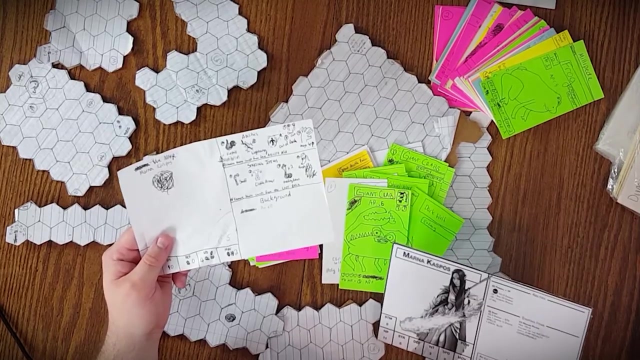 That is what I would call a beginning prototype or testing prototype. We could talk about more of a professional looking prototype And in fact I kind of give you a little a little who's a. what's it right here? This is beginning prototype material, right here. 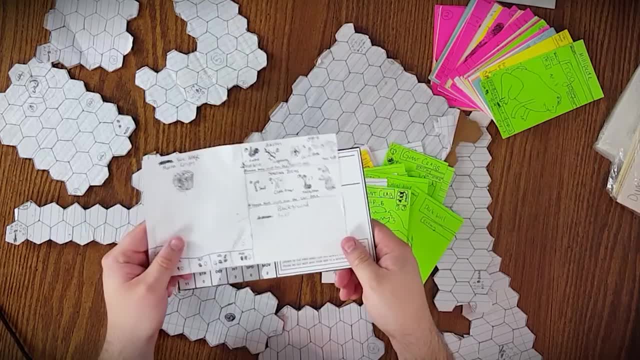 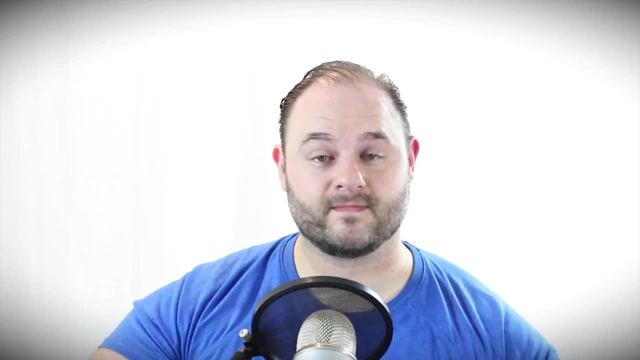 This is end Prototype material. It's actually funny enough, the same character, But, as you can see, the stats and things have all changed because, well, testing is good, Prototyping is good. That's why we're talking about this. 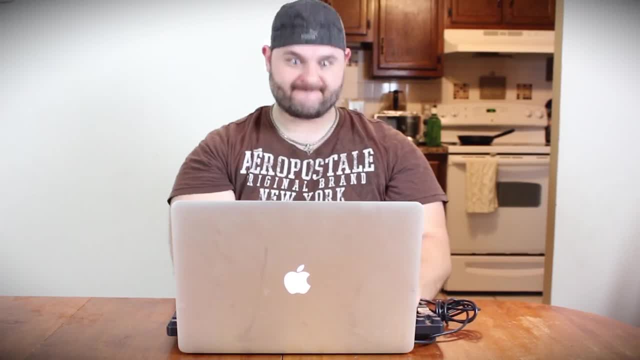 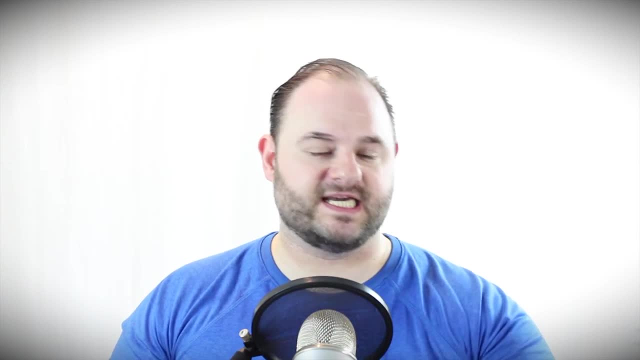 That's why you need to create your prototype as quickly as humanly possible. Get it on the table, Rope your friends into it, Rope your mom and your dad, your kids, your cousins, your uncles. your just grab that bomb off the street. 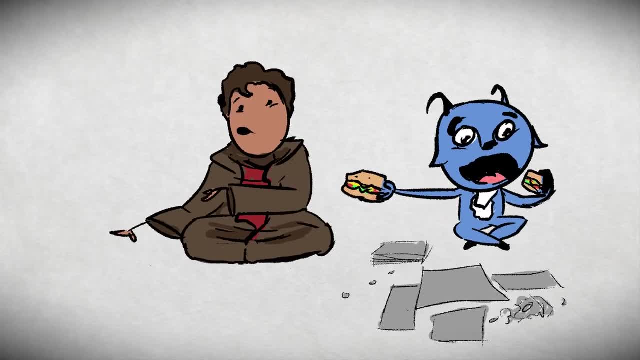 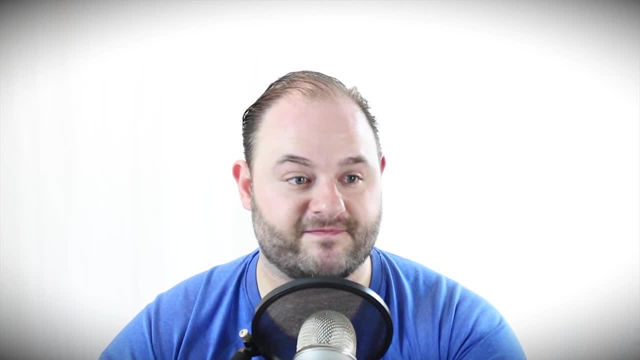 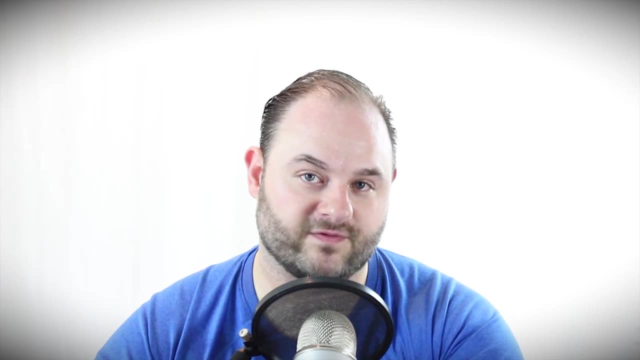 And just hug him and just say, hey, we're going to eat a hamburger and play my board game And he would be like awesome. Recently I found another program that is going to save quite a bit of time for myself and hopefully for you as well. 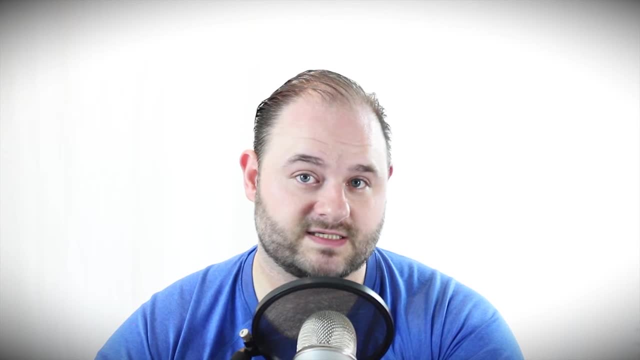 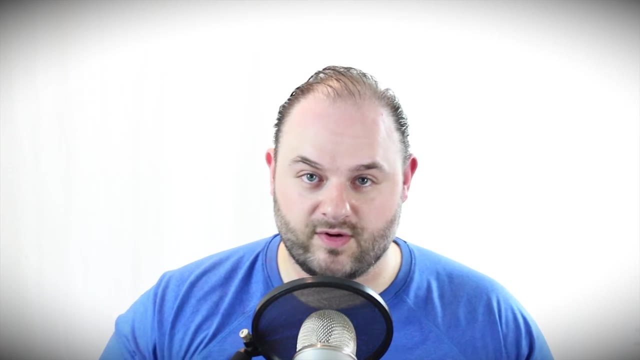 Now, it is free software and I would highly suggest that you donate because it is free, but it's going to save you a ton of time. I'm going to go ahead and show you this, The software that I'm talking to you about. 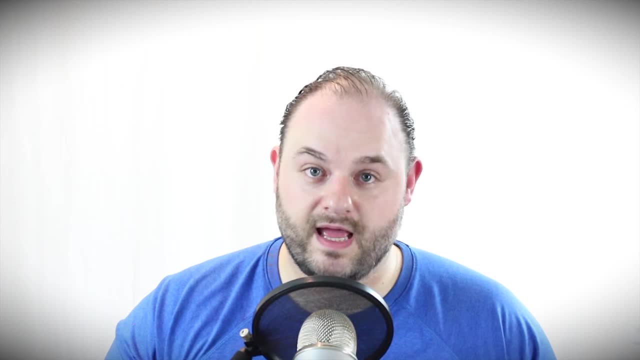 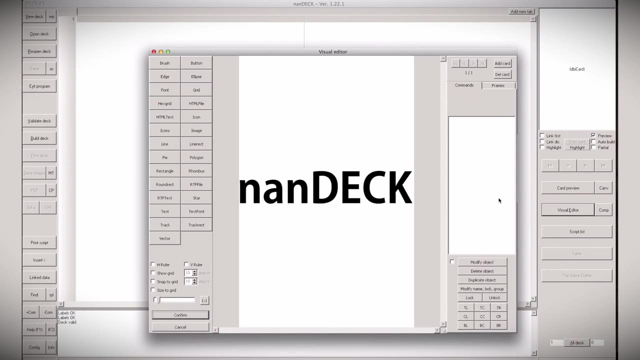 And let's go ahead and move on over to the computer. All right, We are on the computer here and the software is called Nandec. Now there are some tutorials online that you can use to get all of this set up, But let me just tell you that all you need to have is an Excel spreadsheet with all of your data on it. 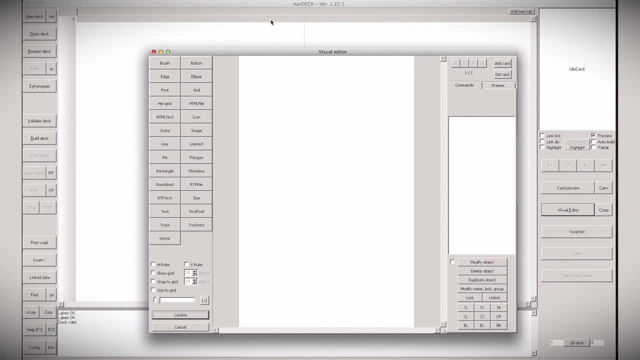 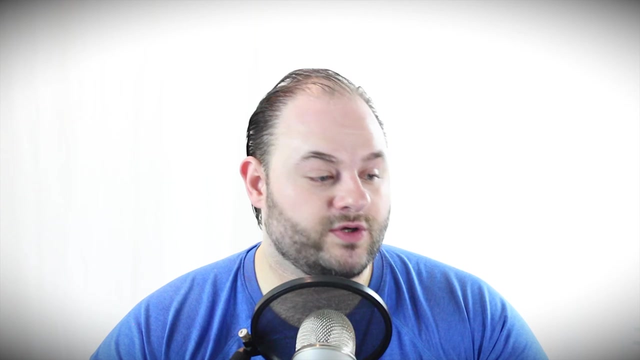 You can configure this program to automatically create however many cards that you have. Now. this program will create your cards for you as quickly as you can come up with them. In fact, all you have to do is write them out in an Excel spreadsheet. 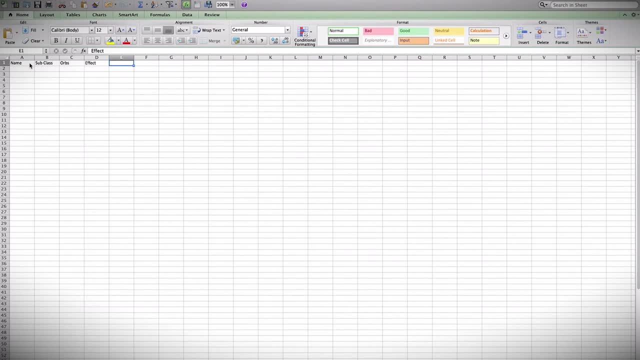 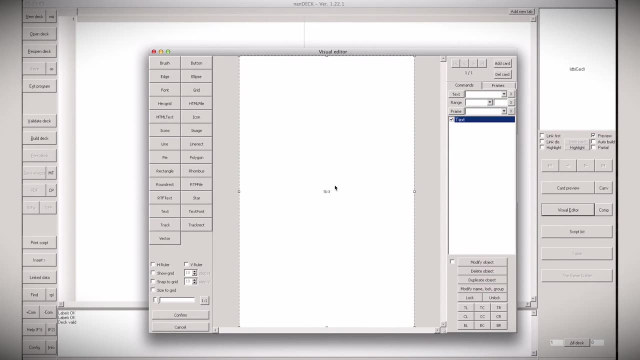 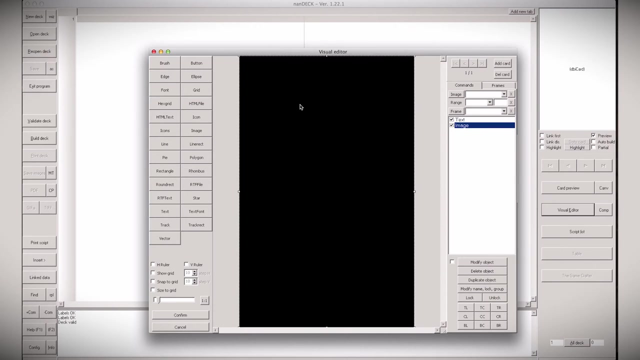 And this will import all of your data and create the cards from a template that you can see right here. I would suggest going on to the website for Nandec, Download the software, do whatever you need to do now, And I am also working on a Mac here. 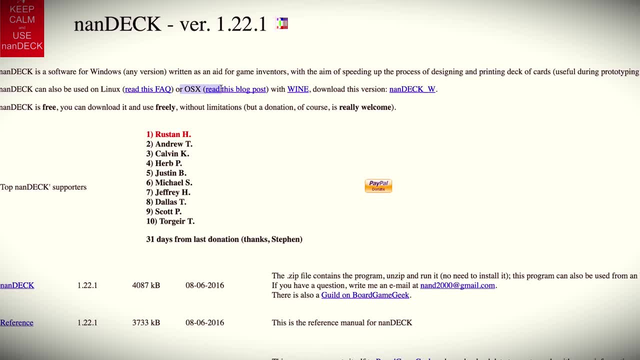 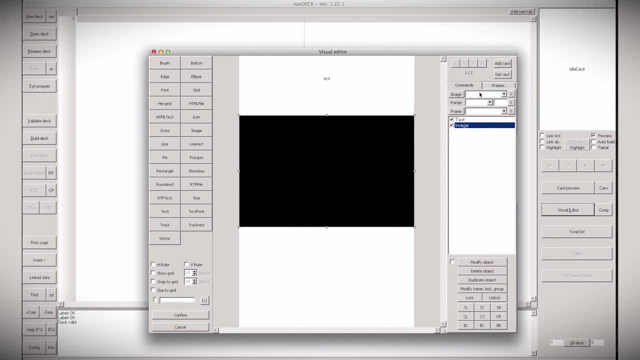 This is actually made for Windows, but you can weasel your way around using some other software to install this exe, which is a program for Windows. Anyways, once you get this program set up, you can enter text, you can alter it, you can do all kinds of fun. 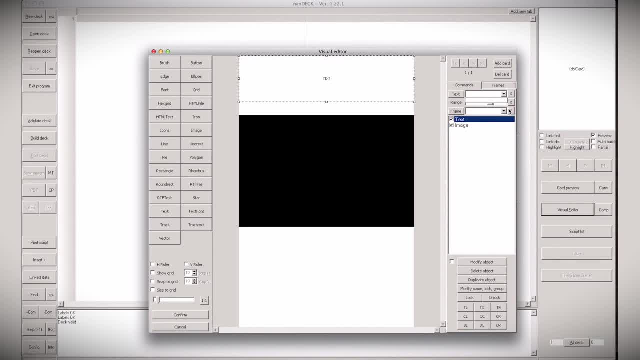 things, Even including adding an image, And what this does is essentially creates a template for you to use. So once this template is made, you can go right on over here, And after you have imported your goodies, you will simply select what this is for.